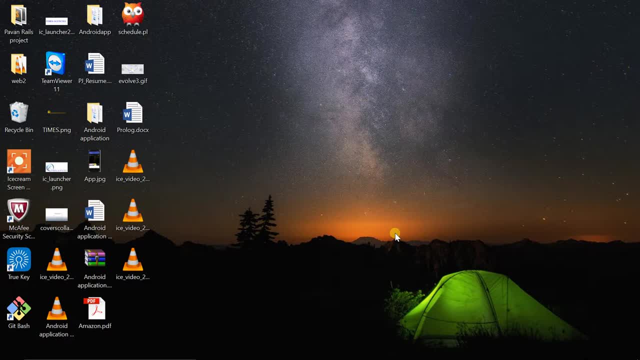 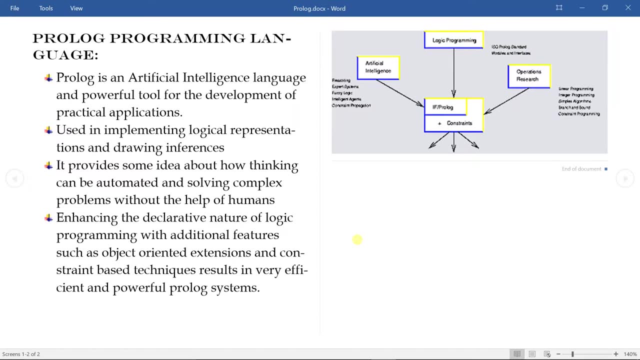 hi guys, here we're going to see compiling, running or writing some basic code in prologue. Prologue is a logic programming language used in artificial intelligence and for checking syntax as well as semantics of a web application, and it also helps in automating human thinking and solving complex problem. 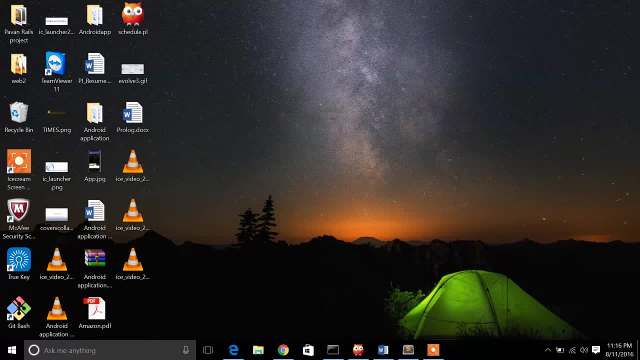 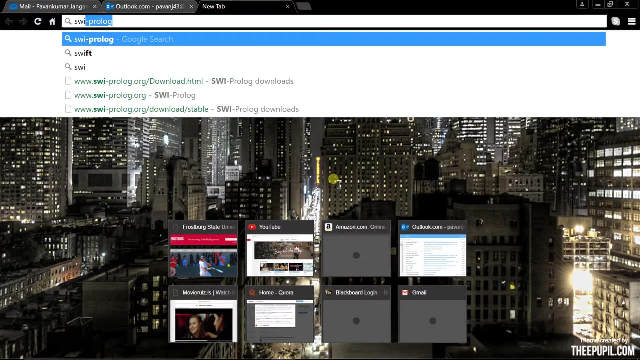 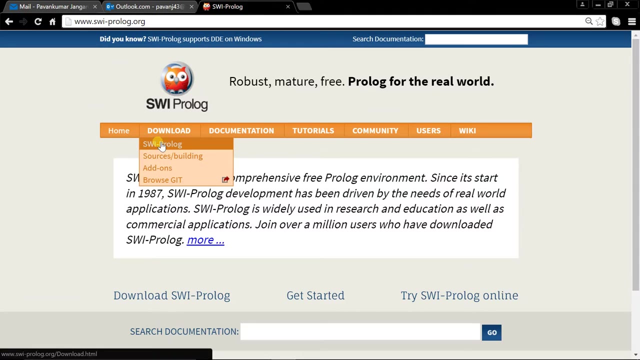 with the help of humans. so I'm going to use a minimal prologue compiler. so I'm use swfprologue. Swfprologue is used for implementing Prologue programming language. download swfprologue. I have a 64-bit version of operating. 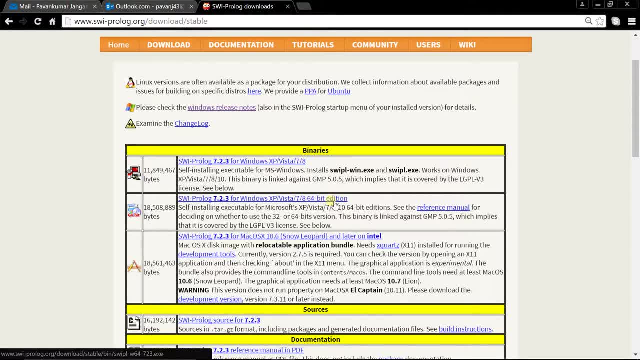 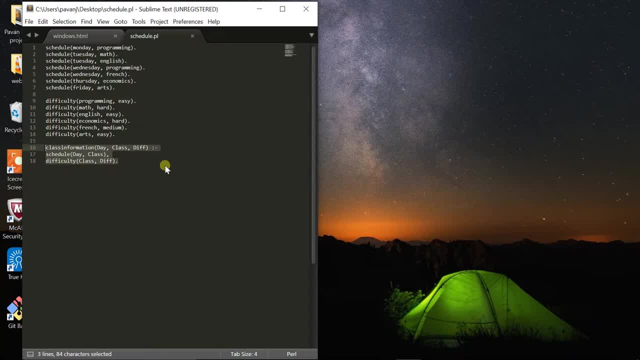 system. so I'm downloading 64-bit edition compiler. so once you're done- done with downloading and installing your compiler- you go for the programming part. these are code I have for my prologue. so these are a school schedule and have different courses, but this is called a fact, called schedule and have a. 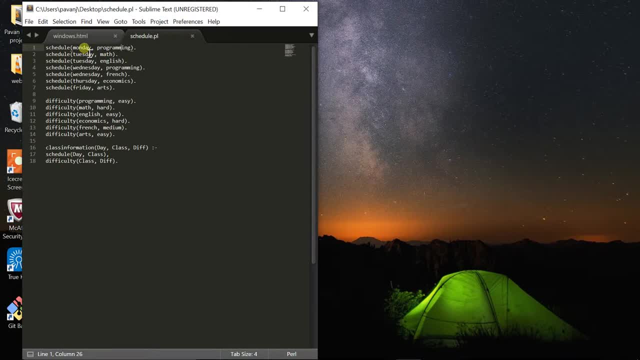 day and the programming course. so on Monday I have programming, Tuesday I have math and English, Wednesday I have math and French, Thursday I have economics and Friday I have arts. so on this part I have defined the difficulty level, like which code is hard, easy and medium. so on this part of the code retrieves. 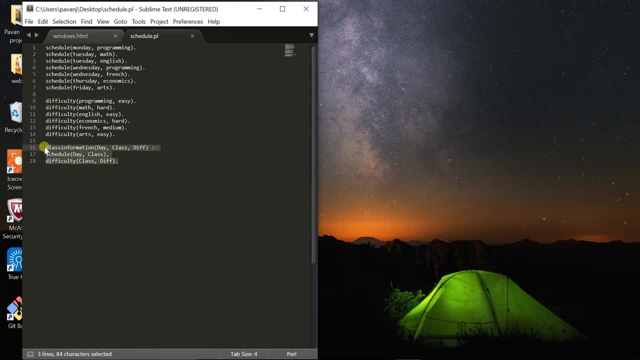 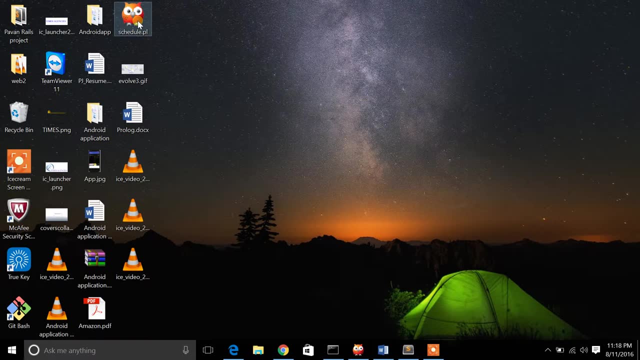 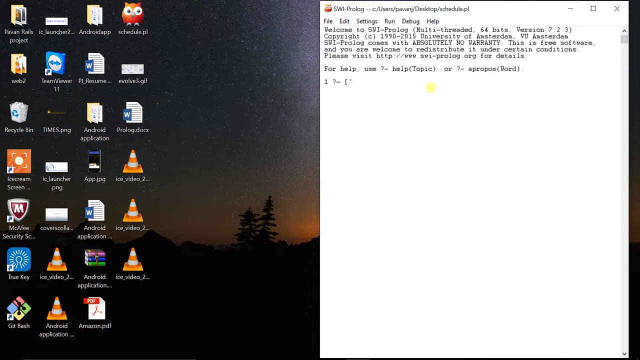 information from a schedule and tells me which codes is difficult and which course is easy. so now I want to compile my code for that. I want to open my source code with SWI prologue. so open our left bracket and a single code and I want to find the source path of my code. 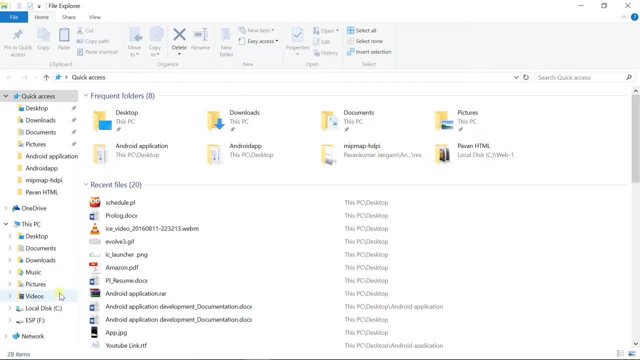 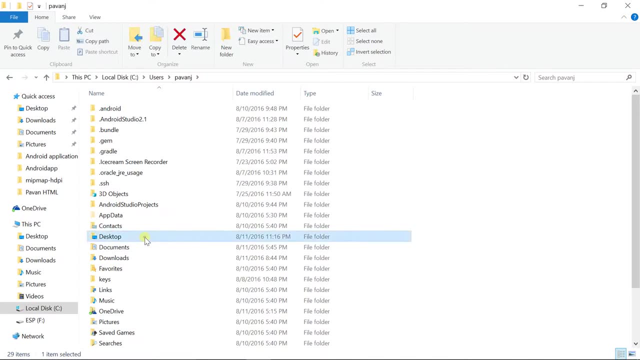 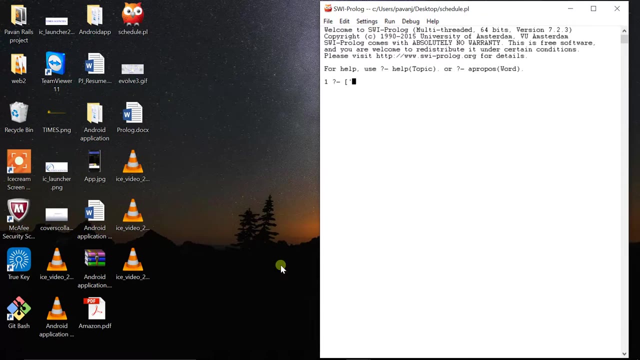 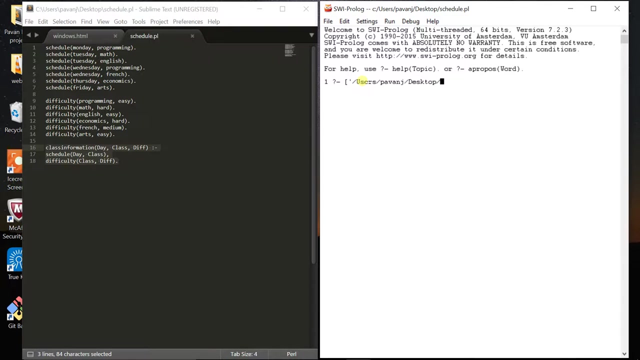 my source code, the C Drive users desktop. so here's my source code file. just copy the path, just paste it here. use the name of your file here so that we'll represent the prologue code, enter full stop and enter. so my code runs with no errors. so now I want to. 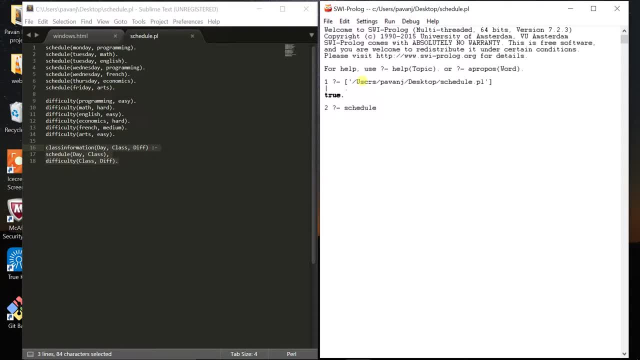 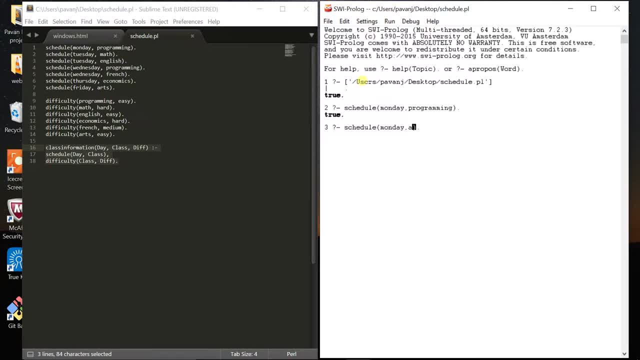 Monday. what if I say I have arts on Monday, so false. I don't have a class on Monday. so I want to check it. difficulty level of my courses: you difficulty, difficulty programming. so I want to see if my programming course is easy. this is true. add my. 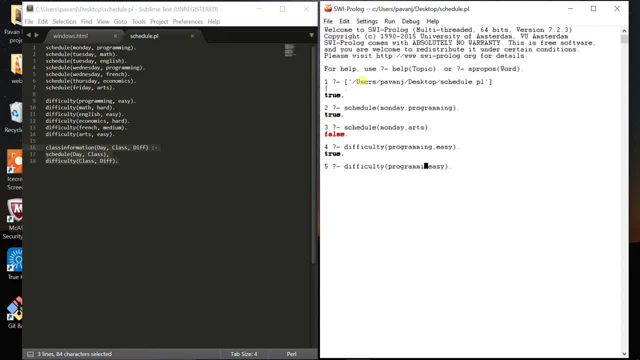 programming code is easy, but if I see my math coach is easy, I'm a fag in math easy. 惜 isch auf sie, die ne l fiquei im easy variables, so my math code is difficult. so i want to check the class information from my schedule and my difficult and easy courses. 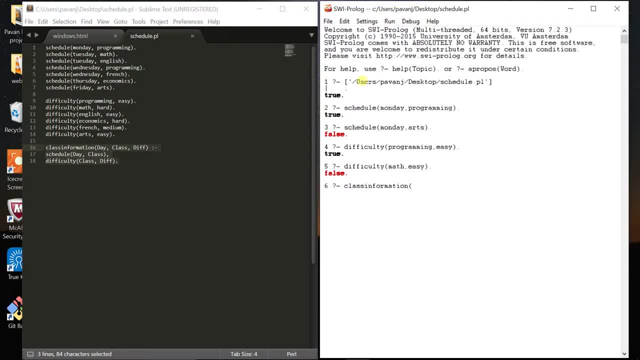 so here i'm taking my class information on tuesday, what classes i have and what's the difficulty level. so on tuesday i have a math class which is hard. you also have a english class which is easy. so let me check what are the all the easy classes i have.